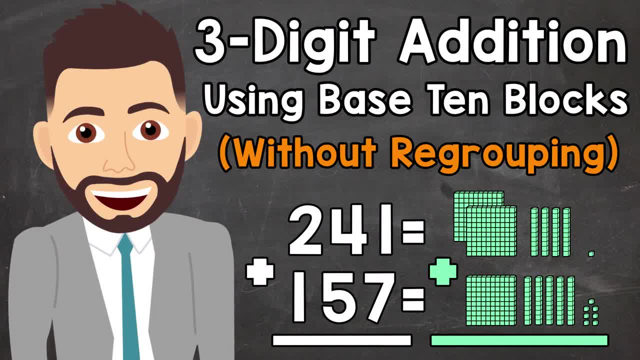 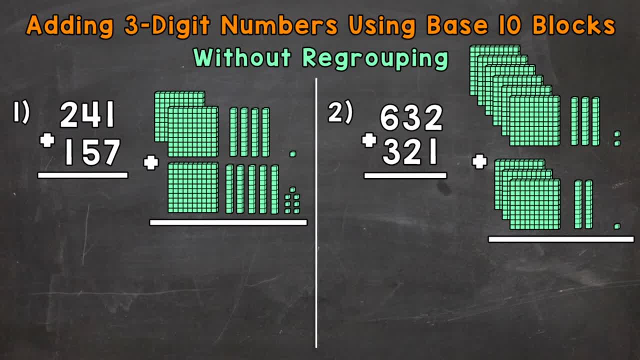 Welcome to Math with Mr J. In this video, I'm going to cover adding three-digit numbers using base 10 blocks. These problems are going to be without regrouping. Now, using base 10 blocks is going to help us visualize what's going on within these problems and give us a better 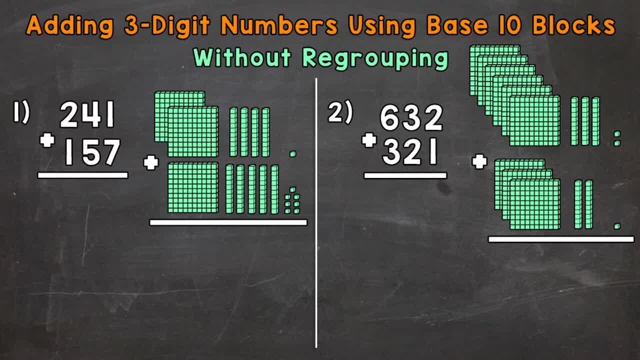 overall understanding of addition. So let's jump into number one, where we have 241 plus 157.. Both of those numbers are represented by base 10 blocks to the right of the problem. Now, when we add, we're going to start with the ones place. So we have 1: 1 plus 7 ones. 1: 1 is 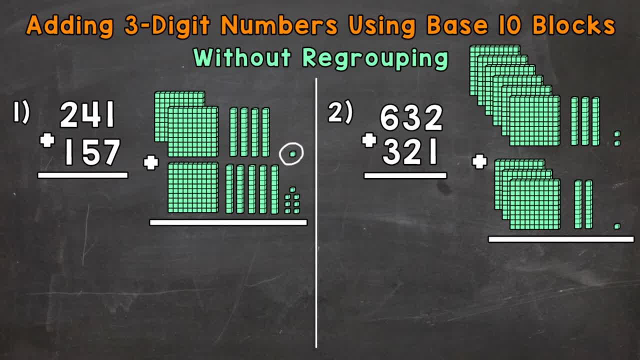 represented right here from the number 241, and then 7 ones from the number 157 is represented right here. So 1 plus 7 is going to be the number 157. Now when we add we're going to give us a total of 8 ones. Now we work our way to the left So we have the tens place. 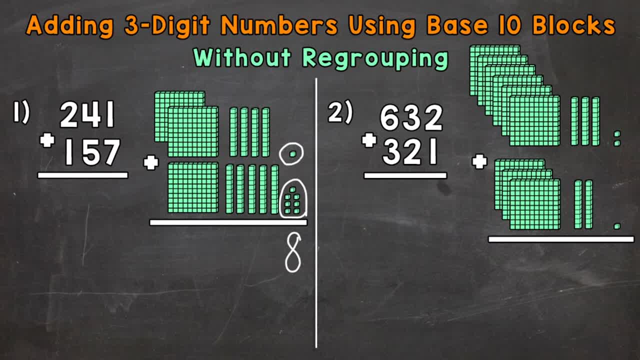 next We have 4 groups of 10 plus 5 groups of 10 or 40 plus 50. So 4 groups of 10 is represented right here, because in the number 241, we have a 4 in the tens place. That represents. 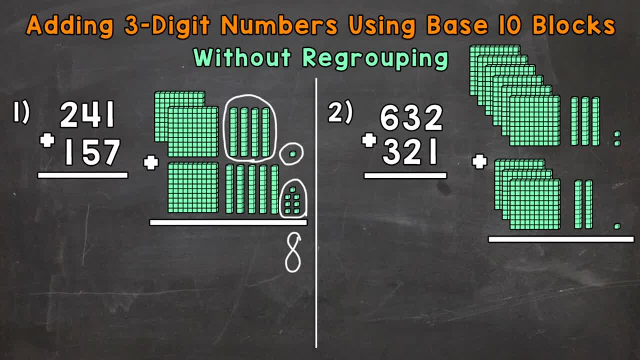 4 groups of 10 and has a value of 40. In 241, we have a 5 in the tens place. That means we have 5 groups of 10 and that's represented right there. That 5 has a value of 50. So 4 groups of 10 plus 5 groups of 10 gives us. 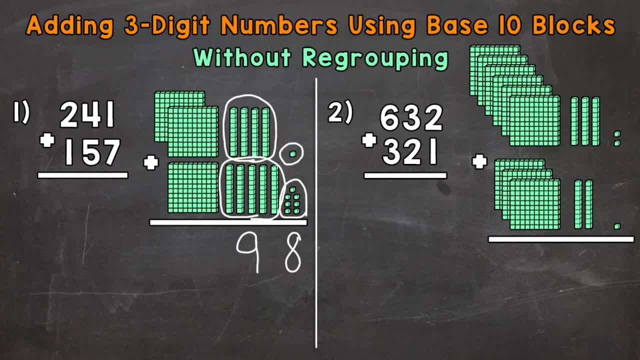 9 groups of 10.. And that 9 has a value of 90.. Lastly, we have to add the hundreds place. So in 241, we have a 2 in the hundreds place. That means 2 groups of 10 plus 5 groups of 10 is represented right here, So 4 groups. 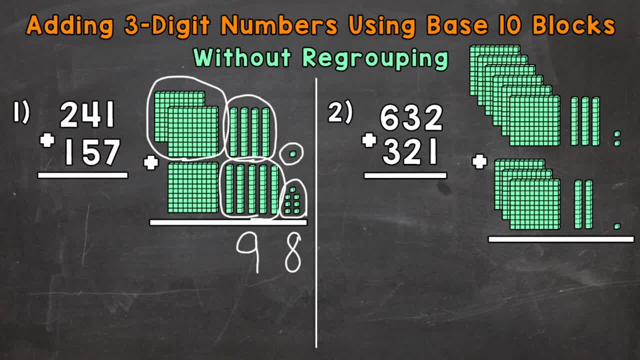 of 10 plus 5 groups of 100, and that has a value of 100.. Now in 141, we have a 6 in the tens place. That means 4 groups of 10 plus 5 groups of 10. That mean 1 group of 100. so we chopped s 0 and our answer is 1.. 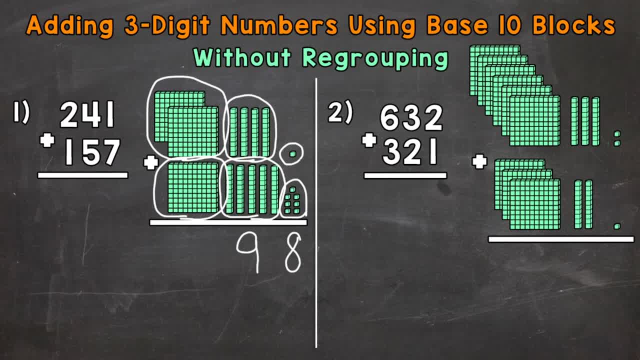 That 1 is represented as a 1, because it's in the hundreds place and represents 1 group of 100. So 1 group of 100 plus 2 groups of 100 equals 3 groups of 100. That's how many. things we have. Okay, this is 1. We have another 10 group of 100. That means 2 groups of 100. So 1 group of 100 is represented by 3 groups of 1 hundred. That would be a 2. 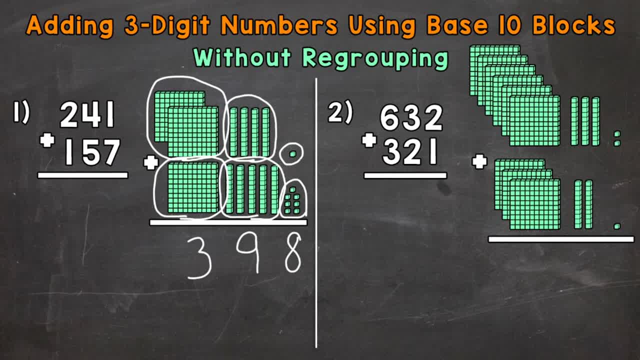 has a value of 300. So our final answer is 398.. To recap, we did 1: 1 plus 7 1's. that gives us a total of 8: 1's. Then we did 4 10's plus 5 10's. that gives us a total of 9 10's. And then 2 100's. 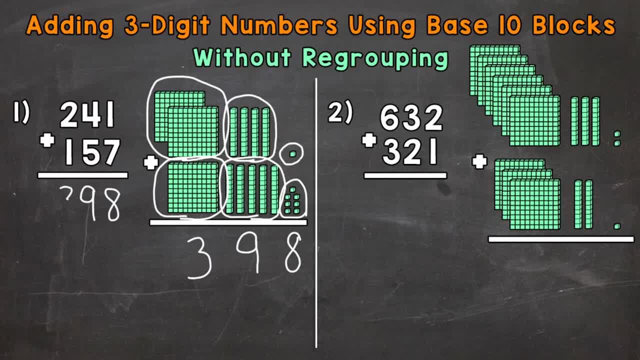 plus 100 gives us a total of 3 groups of 100, and that has a value of 300.. So final answer: 398.. Let's move on to number 2, where we have 632 plus 321.. And we start with the 1's place. 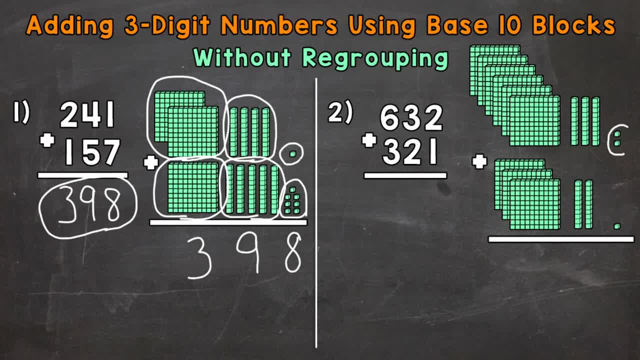 So 2 1's from 632 plus 1 1 from 321.. That gives us a total of 3: 1's. Let's move to the 10's place. So we have 3 10's or 30, plus 2 10's or 20.. 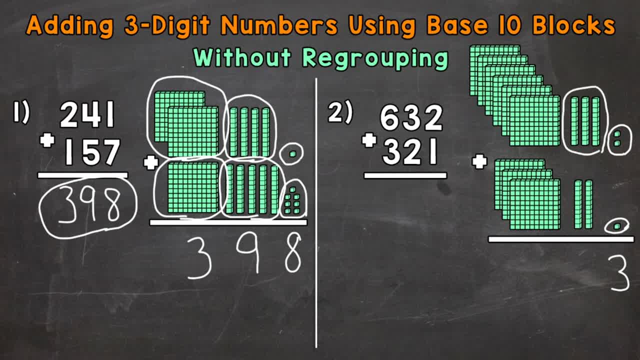 3 10's plus 2 10's gives us a total of 5 10's or 50.. And then, lastly, we have the 100's. So for 632 we have a 6 in the 100's place. That represents 6 groups of 100 and can be seen. 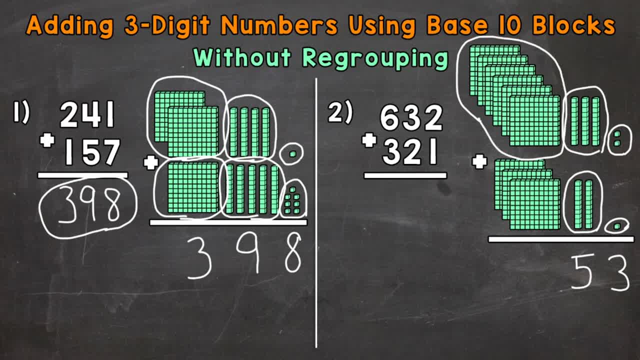 right here: 6 groups of 100.. That has a value of 600.. Now for 321. we have a 3: 1's place. That represents 6 groups of 100.. That has a value of 600.. Now for 321. we have a. 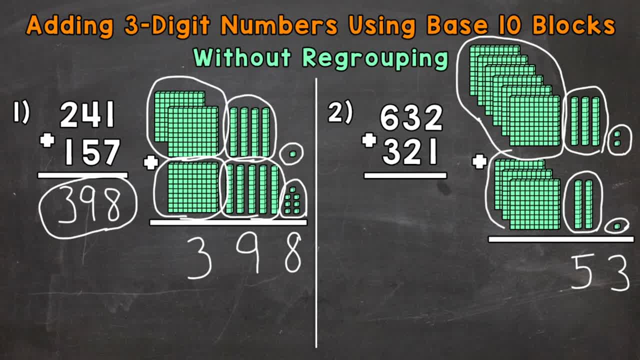 3 in the 100's place. That represents 3 groups of 100 and has a value of 300.. So 6 groups of 100 plus 3 groups of 100 gives us 9 groups of 100, or a 9 in the 100's place, And that 9 has a value of.